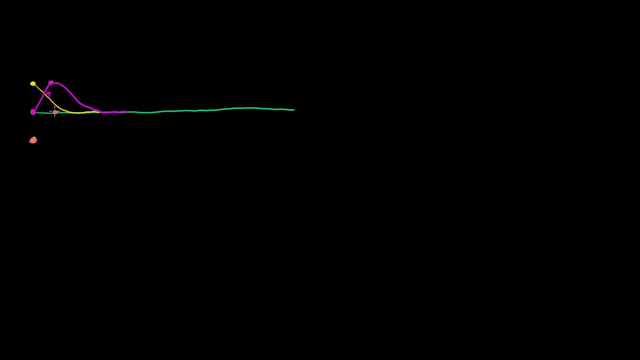 And now he's going to switch directions And he will have gotten here at that point, The point on the line that was here, I guess on the purple period of time it had some upward momentum, So it's just going to keep going, maybe at a slower. 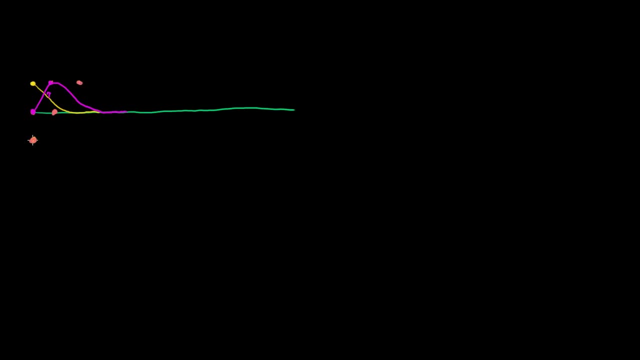 pace and it'll be there And it'll bring the rest of the rope to the right of it with it. So now my rope is going to look something like this, And then, finally, Where I'm going to jerk the rope back to: 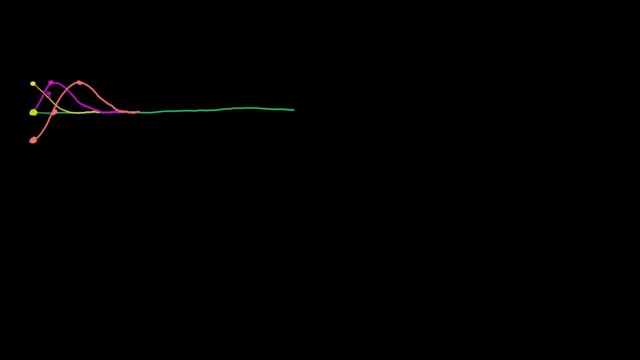 its original position. So this left-hand point's going to be there. When the left-hand point is there, this guy in the previous time period was moving down rapidly So he might get there ready to switch directions again, This guy will start moving down. 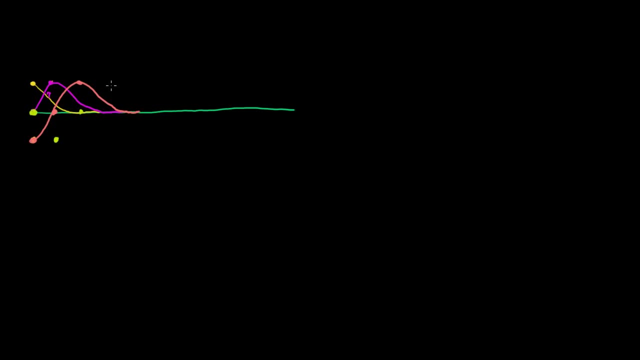 This guy right here. he had some upward momentum, So he's going to be up in this position now And he's going to be ready to switch directions. So finally, when I've done this whole cycle, when I've moved up, down and back, there again my rope might look. 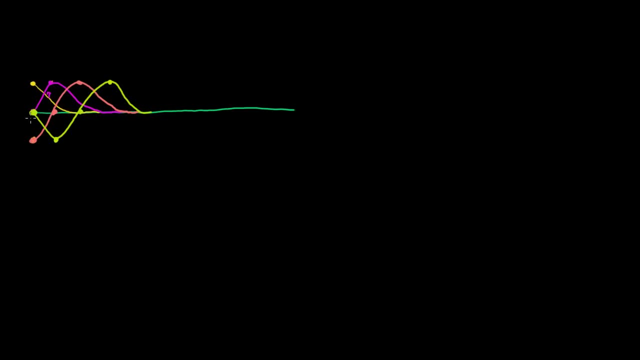 exactly like this And I could let go of the rope. I could just leave this little left point right there And this lump is going to propagate along the rope, Because in the next moment of time, what's it going to look like? 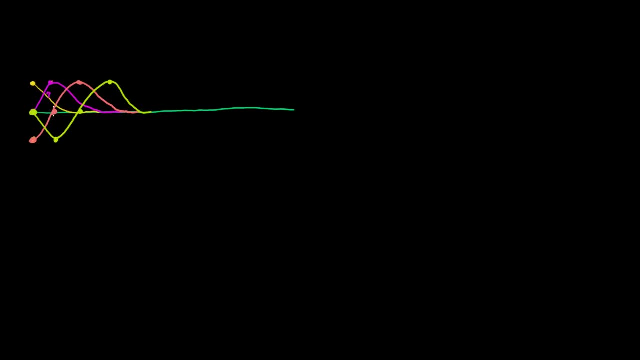 This guy is going to be pulled up by this left-hand point, So he'll go back to his resting position. This guy's being pulled down right here by the part of the rope to the left of him, So he's going to be pulled down. 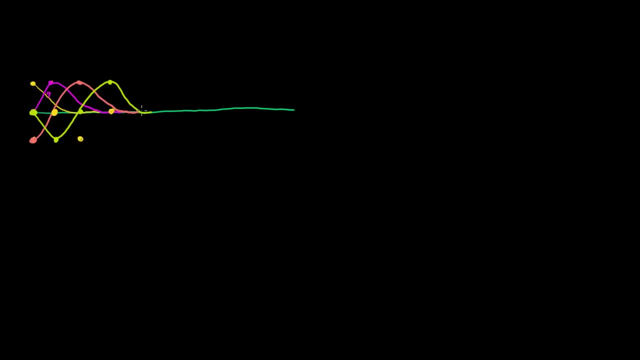 This guy's being pulled down, But this guy had some upward momentum in the time period before, so he will have moved up. And so in the very next time period, my rope is going to look something like this: And this disturbance in the rope, if I do nothing else. 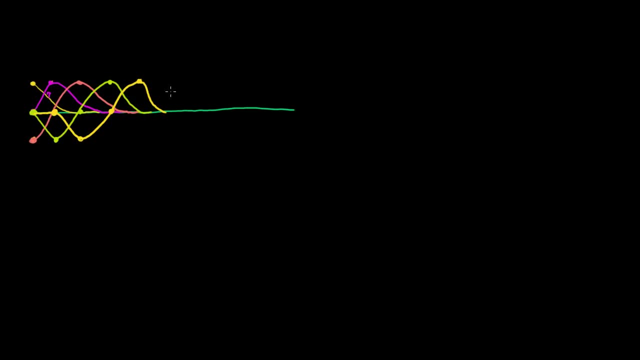 and if I don't lose energy to heat and friction and all of that, it'll just continue moving down the rope. If I look at the rope at some future period in time- maybe not that far down- the rope- will look something like this: 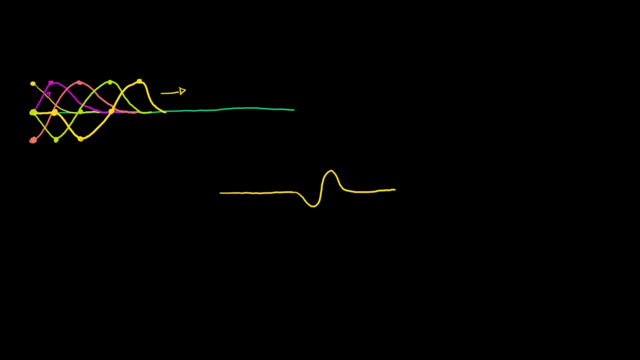 And if I were to keep watching it, I'll see this disturbance. I keep using the word disturbance because there's really no better word to use for it. I'll see this disturbance, or perturbation, or whatever you want to call it, moving along the rope. 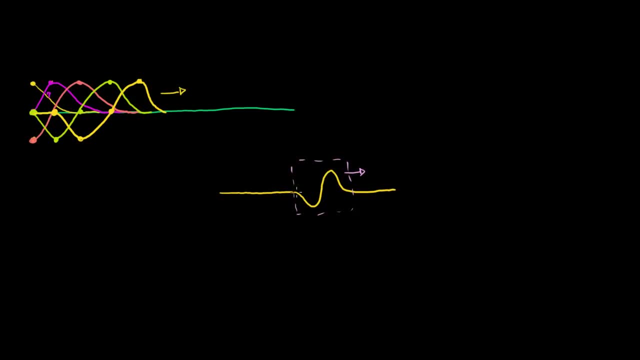 And so when we think about what a wave is, we essentially- I kind of jumped the gun. I keep calling this a disturbance because I didn't want to use the word wave. I want to say, well, what really is a wave? 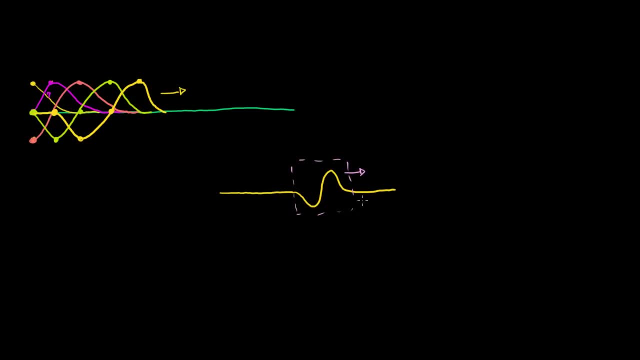 And a wave really is just this disturbance that's propagating down the rope. So this is a good time to actually define a wave, Because once I define it, I can start calling this a wave as opposed to a disturbance propagating down the rope. 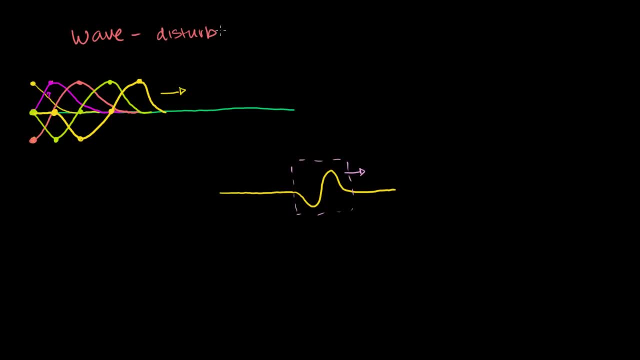 So a wave is a disturbance propagating through space, And you might see other definitions of a wave. One of the most typical ones, A disturbance, is energy or a disturbance propagating energy through a medium, And when they say medium, it's what is the wave going through? 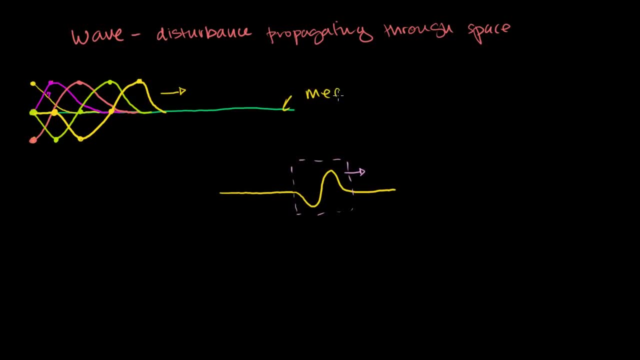 So in this example the rope would be our medium. But the reason why I don't want to use that definition of a wave is because in future videos we'll learn about electromagnetic waves, And those don't propagate through any medium, They propagate through a vacuum. 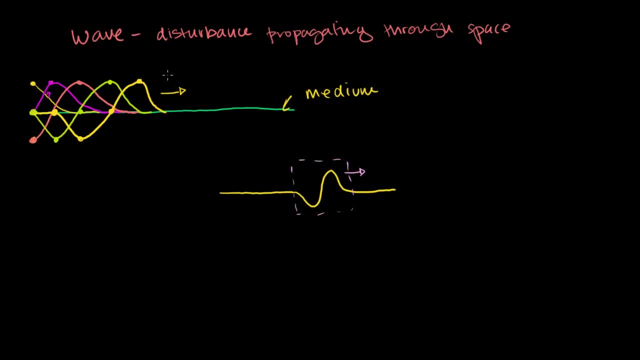 So, to keep things as general as possible, we'll just call it a disturbance that propagates through space, And it usually transfers energy. What do I mean by transferring energy? Well, on this left-hand part of the rope, I gave a little. 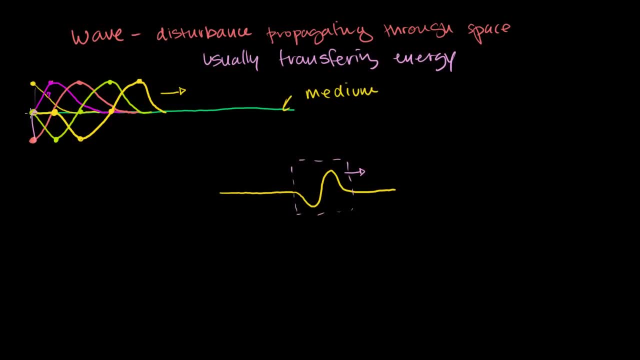 energy to the rope. I moved it up down and then back again And then, after I did that, that up down, back again is happening successively to every point to the right on the rope. So if I wait long enough at this point on the rope right. 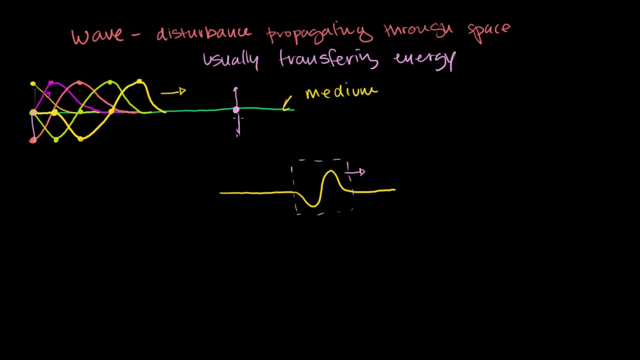 here it's going to move up, down and then back again. Exactly what I did over here is going to happen to this point on the rope And then later on it's going to happen to some other future point on the rope. 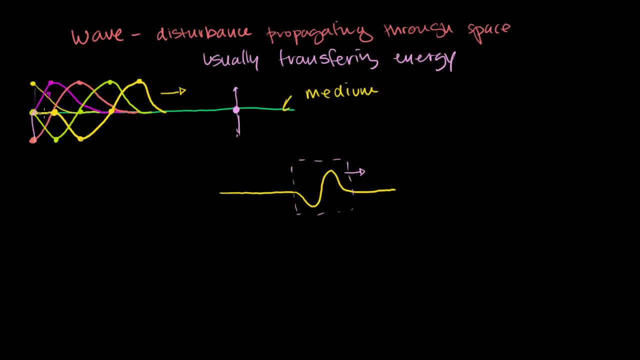 So that energy that I originally put in on the left-hand side of the rope is being transferred down the rope. If I had some type of object here sitting on the rope, maybe when the wave, when the disturbance passes through the rope, when the disturbance passes by it, this thing could. 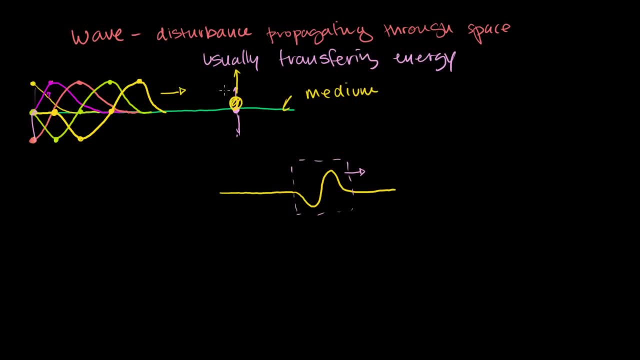 get flipped into the air. It might get pushed into the air and go into a higher potential energy, So this disturbance is transferring energy, in this case. Now, what I've drawn here, this isn't the only type of wave you can have. 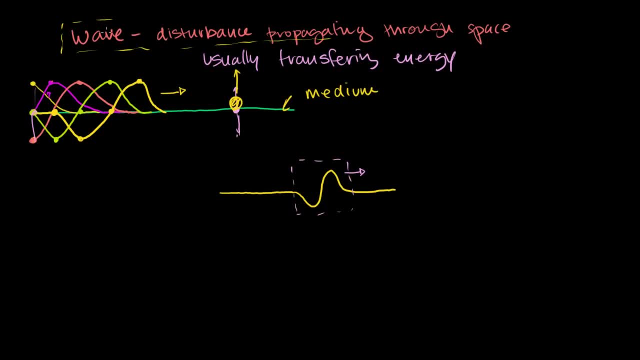 I mean, my definition is fairly general. But the definition is more general than just what I've drawn here. For example, you could have a sound, wave A sound. imagine you have a bunch of you know, if you just look at all of the molecules in the air, they're just you. 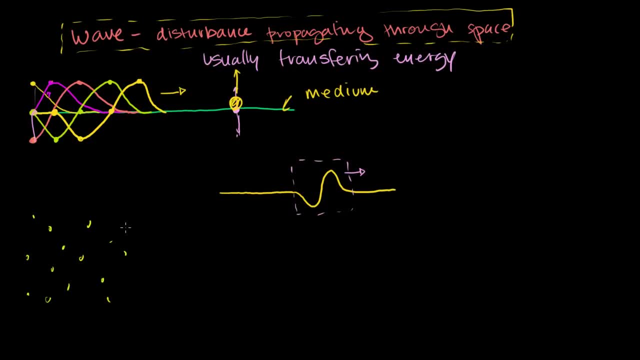 know they have some density. that looks something like that And I'll say I had some type of a membrane. maybe it's a speaker that jolts this left-hand side of the air So it just pushes. So let me see if I can draw this. 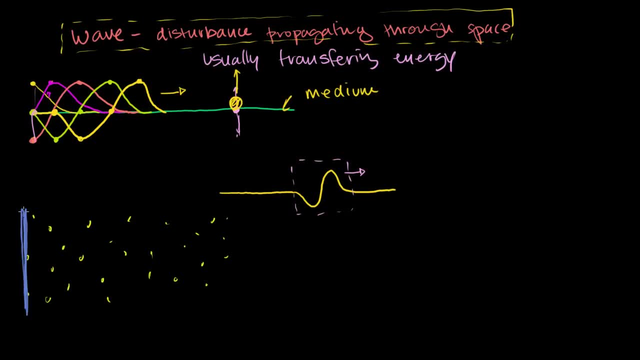 So let's say, I had some type of surface here that just really quickly jolts, that just moves in that direction and then just comes back. So just similar to what I did here: I go up and down, But instead of doing that it just pushes the air and then 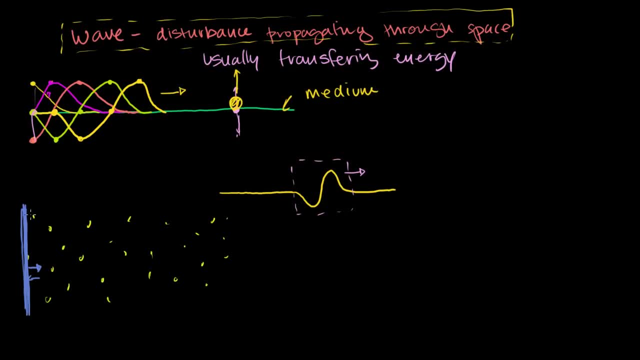 pushes back. So what's going to happen? So, right after it pushes it, the air molecules that it pushes up against are going to jam together. They're going to get compressed right here. All of these air molecules that were right on the surface are 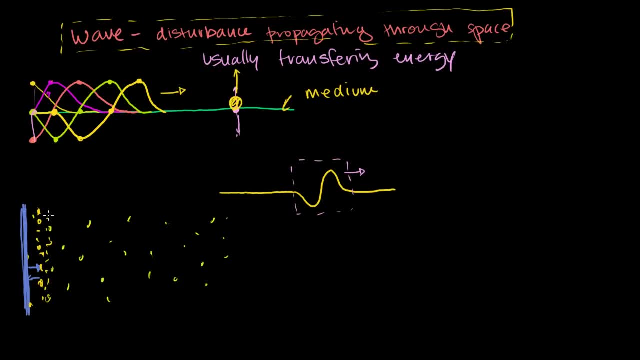 going to get pushed next to all of these air molecules that are right there, And then when it pushes back, or when the membrane goes back, you're going to have fewer air molecules here because you're going to have a low density here. And then these guys, they're all squenched up. 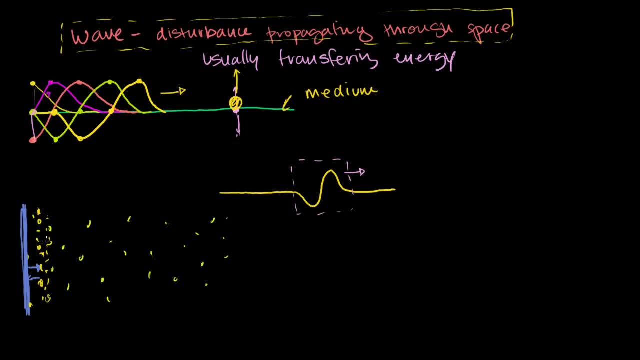 together. They're going to want to get away from each other. They might even run into each other, And so these guys are going to run into those guys, who are going to run into the next guys, and so on and so forth. And after these guys bump into those guys, those guys are. 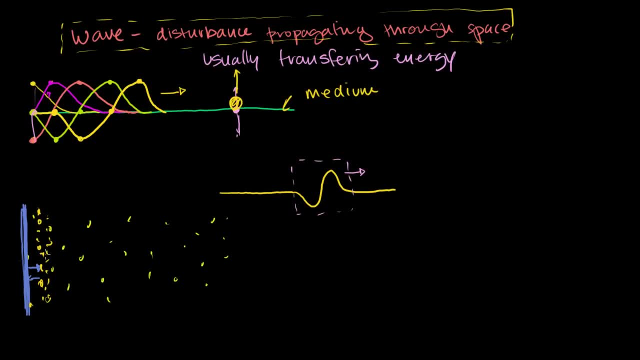 going to go back to where they were. So essentially you're going to have this kind of disturbance: is going to be one molecule bumping into, or a set of molecules compressing or bumping into its neighboring molecules. So if you look at this at some future period in time, all of 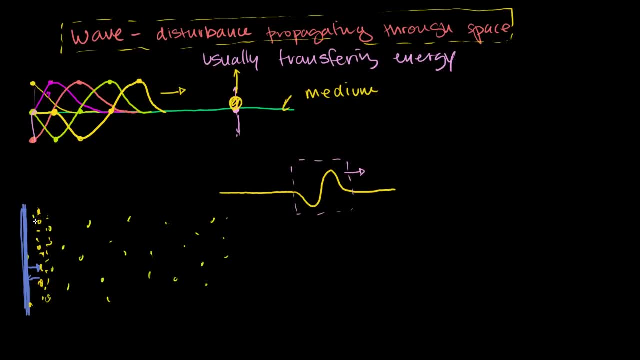 a sudden, this area might look normal. Let me click Clear it and draw it just the way I started off, So this area might look normal. This area will look normal, but that compression of the particles might have reached right over here. 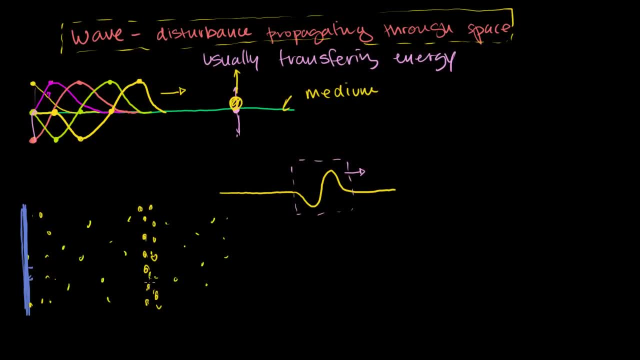 That compression of the particles might have reached right over there. And not only that, we saw that right after the compression you usually have an area of low pressure. So if I were to really draw this wave and actually if this membrane were to keep doing it over and, over and over and 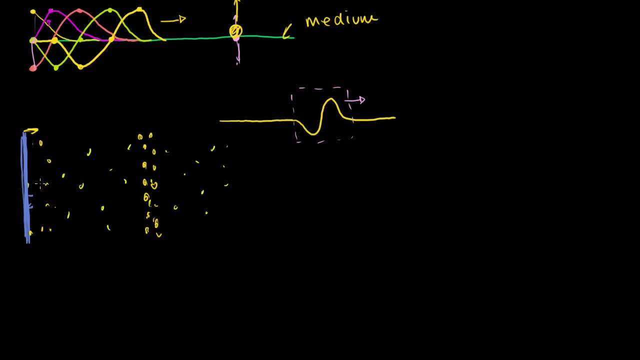 over again. so it kept going forward and back, forward and back, or right and left, right and left. what you would have is a series of compressions. The air would just have a series of compressions. So that's one compression. 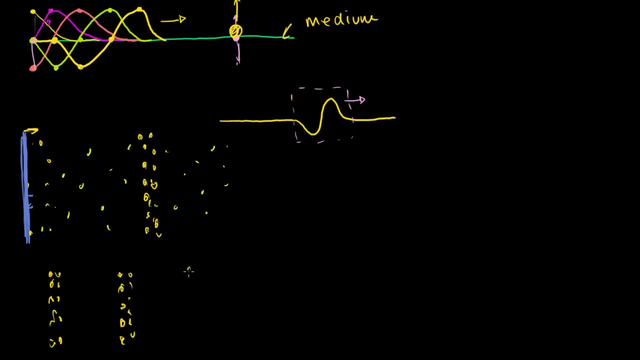 You'd have another compression right there, another compression right there, And then, in between the compressions, the air is less dense, like this, And what we've essentially just generated is a sound wave traveling through air. So this right here, This is a sound wave. 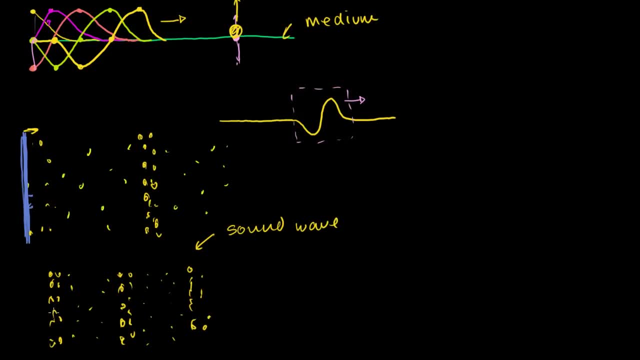 And this type of wave where the direction of the disturbance is the same or along the same axis as the direction in which the wave is traveling. the wave is traveling in that direction. this is called a longitudinal wave. So sound waves sound through air. they're longitudinal. 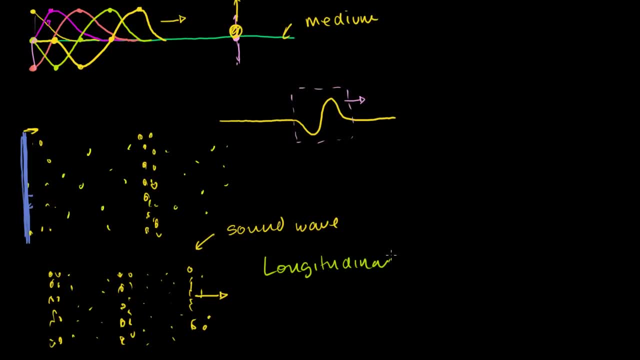 waves- longitudinal wave, sometimes called a compression wave, Same thing Compression wave, Because it's caused by compression, Our example of the string. this is called a transverse wave. This is called a transverse wave Because the disturbance, the movement of the medium is. 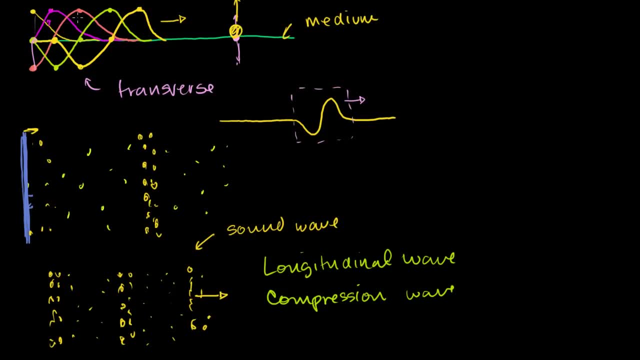 going in a direction transverse to the, or in an axis that's transverse to the direction of our movement. We're moving in that direction to the right, but actually our wave is moving to the right, But the actual medium is moving to the left. 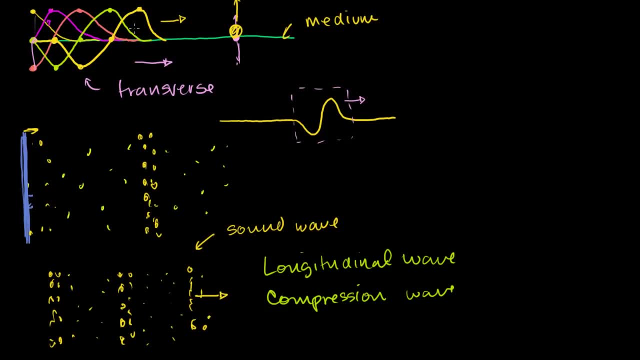 So the wave is moving to the right, but the actual medium is moving to the right. But the actual medium is moving up and down. Our medium is moving up and down- That's why this is called transverse- While here the medium is moving left and right, while 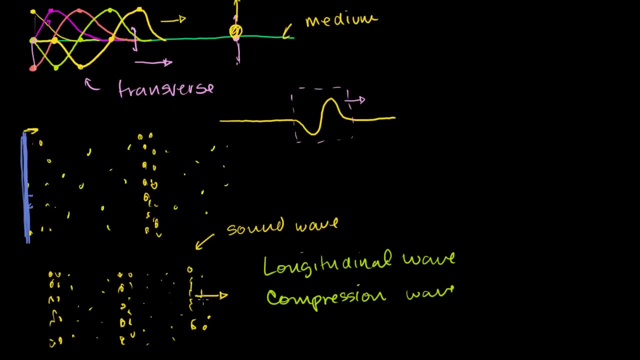 the wave moves to the right, So it's along the same axis. So we're dealing with the compressional or longitudinal. Now, in this first example, I just did one cycle, I just jerked up, down and back again. 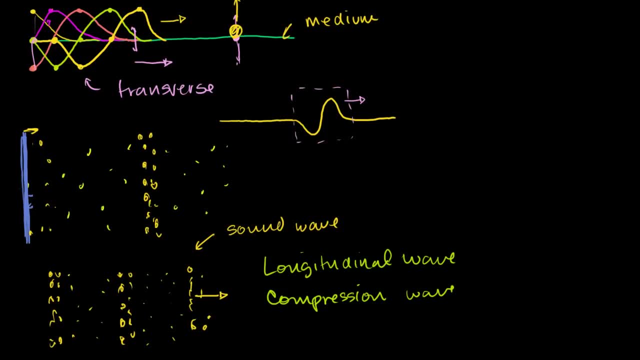 And I created this one disturbance, And we can call this: when you just do it once, you can use this as a wave pulse. If I kept doing that, if I just went up down back again, up down back again, and I kept doing it, 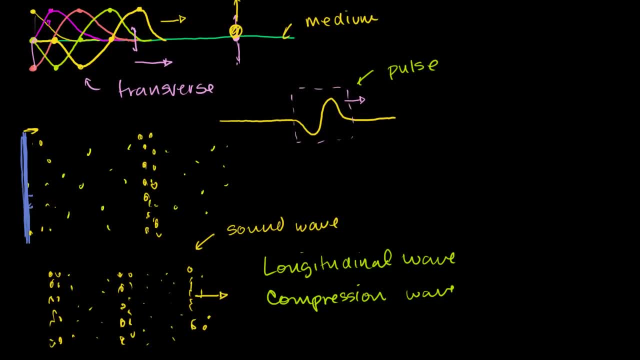 periodically, over and over again. then I would generate a periodic wave And my string would look something like this: Well, actually it would look something like that, right there where that's the disturbance generated from our first time that we generated. 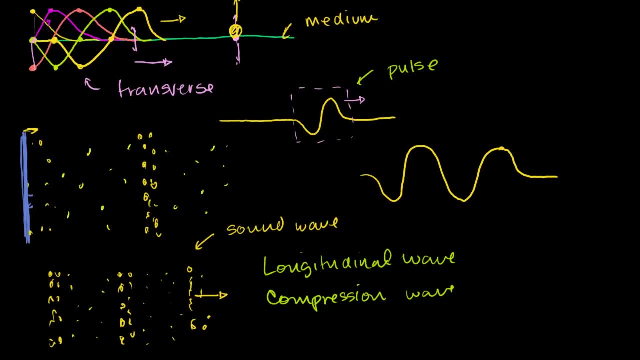 We moved this left-hand part of our string, So this right here is a periodic wave, And in the next video we're going to talk about a lot of the properties of a periodic wave, how the wavelength and its frequency and its period relate to its velocity and all. 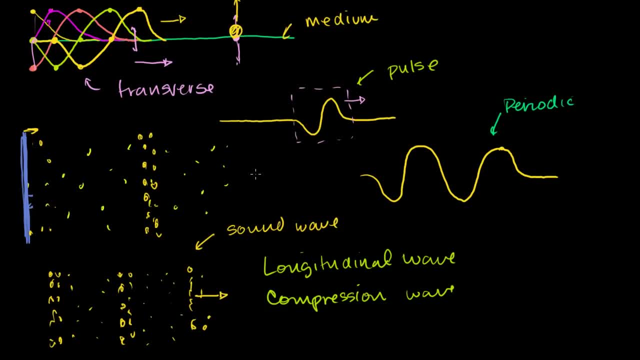 of that, But I'll leave that alone in this video. But I just want you to appreciate what I think is a concept that we use in everyday life. Oh, it's a wave, It's a sound wave and all of that, But it's a fairly abstract notion. 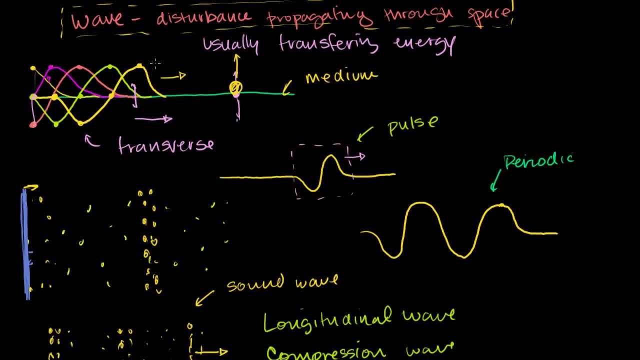 When we talk about a wave, we're really just pointing to a disturbance that's moving, usually along a medium, at least when we visualize it, but not always. But we're just pointing to this disturbance, And the disturbance could take many forms. 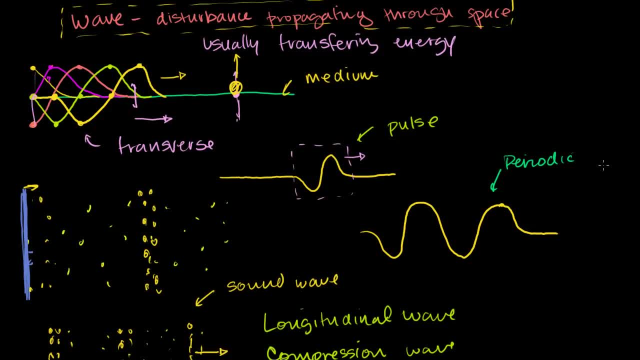 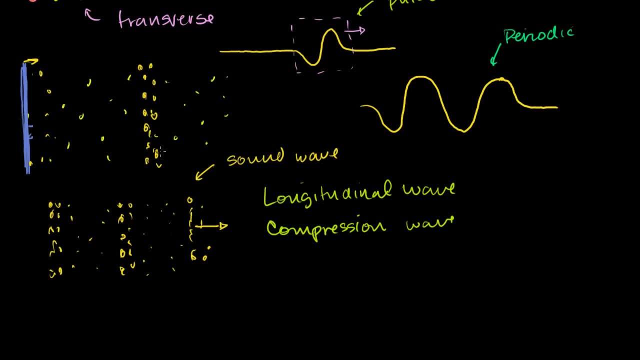 It could be a transverse disturbance. if we're dealing with a string, It could be a disturbance in terms of the density of air molecules, in terms of a sound wave, And there is a relation. So, if you wanted to just plot the density here by position, 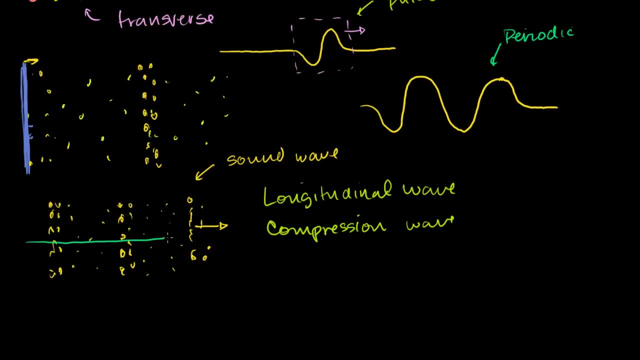 if I were to mathematically represent this compression wave Right Right here. So let's say that this line represents just resting normal before the sound wave hits. That's just your normal density. If we were to plot the density, it might look something like this: 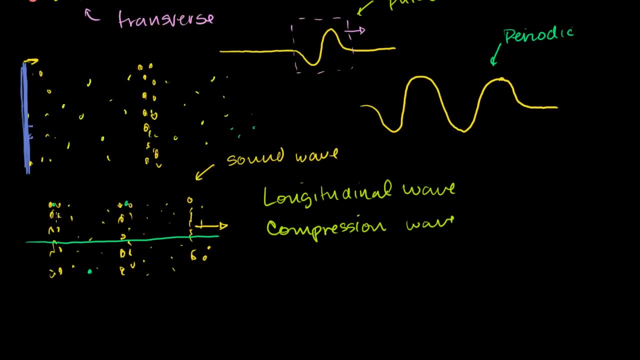 So over here we have very high density. Over here we have very low density. Over here we have very high density. And if you were to plot it, it would look a lot like that transverse wave that I did with the rope. 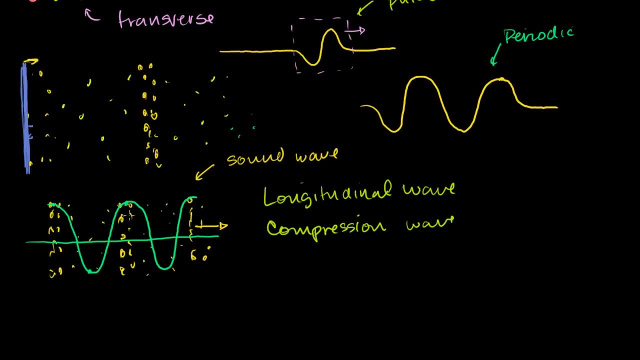 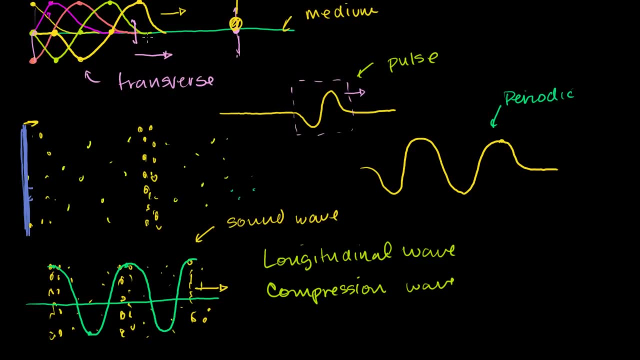 at the beginning of this video. And that's why they're even grouped together, Because, mathematically, even though a compression wave looks very different- or you might visualize it or conceptualize it very different than a transverse wave, mathematically they're essentially the same thing. 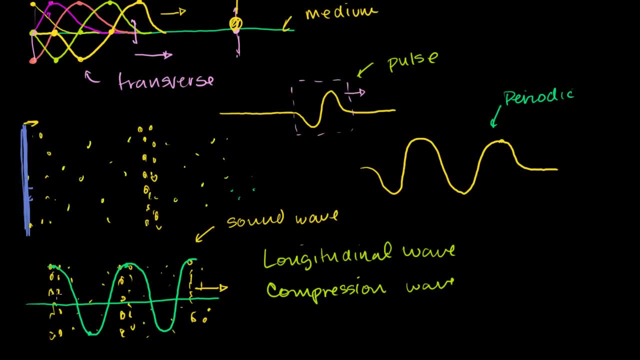 You have this quantity. In this case it's the density of the air varying over time. In this case, it's the height or the position, or how much your displacement from your resting position. That's the quantity varying through time. That disruption is traveling over the course of the medium.